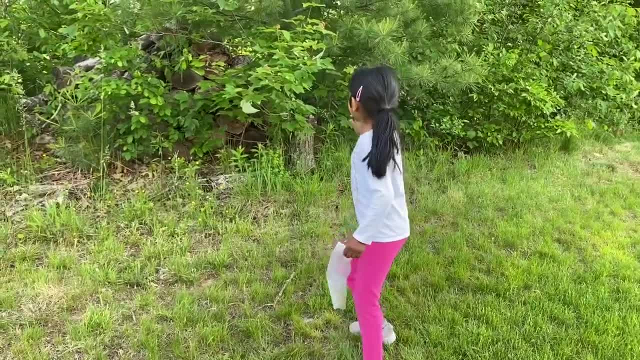 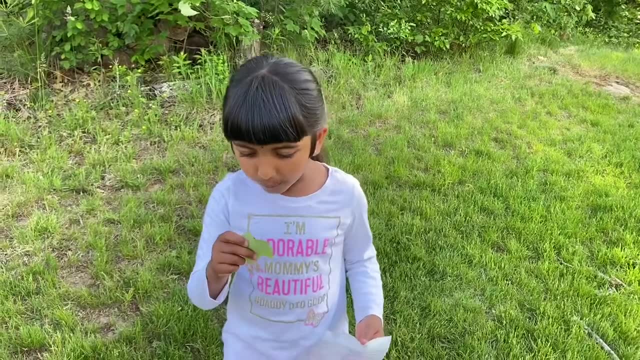 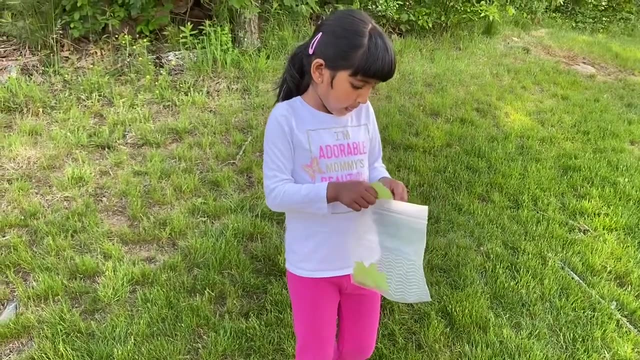 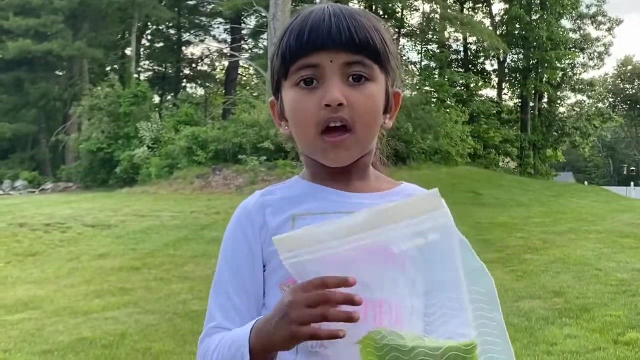 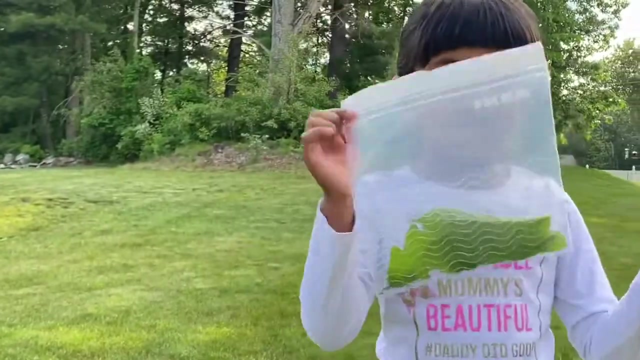 There's two more to find. Let's take it. There's one more. Two more to find Here. I got five different kinds of leaves in this bag. Let's start doing the craft. This is a simple activity. Let's see what we need. 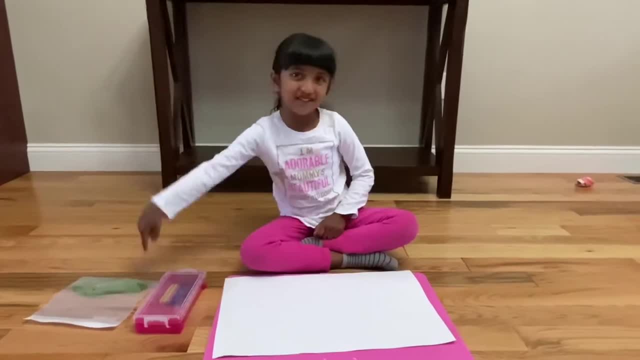 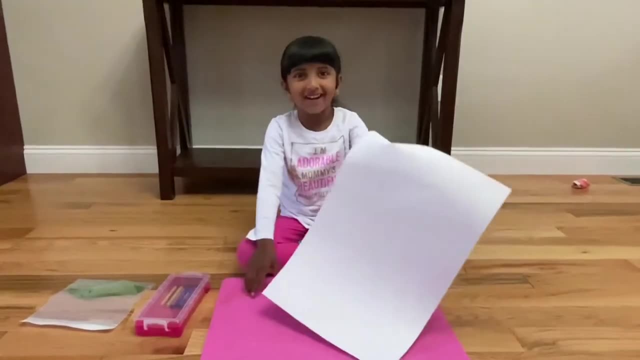 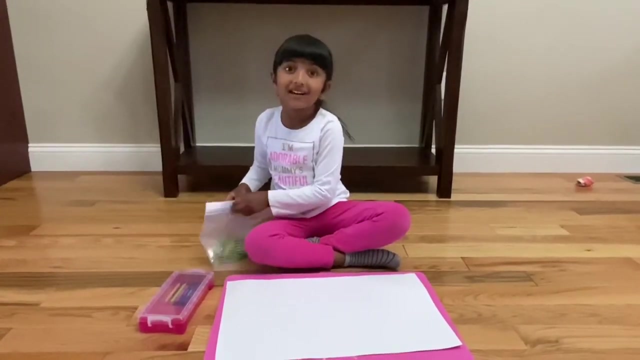 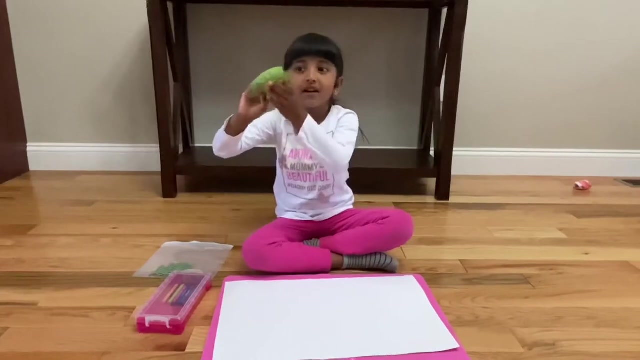 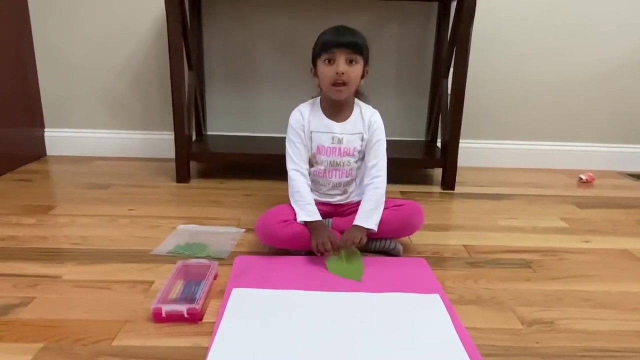 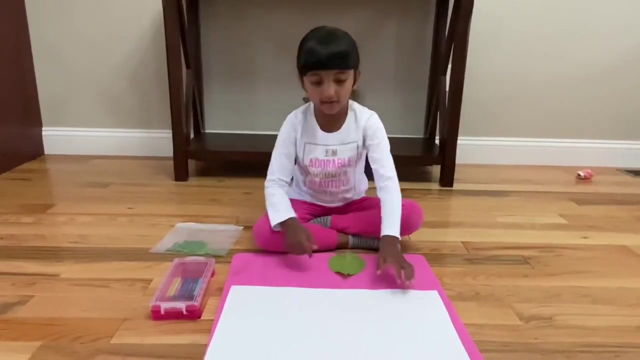 We need crayons, leaves- like we did the nature, one outside and a big construction paper. So I'm going to take one leaf, okay. So first we'll start from the big to small. okay, Let's put the leaf under the paper and on the leaf you feel it and trace it, okay. 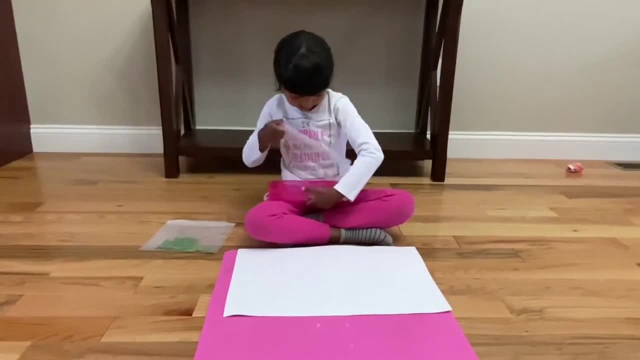 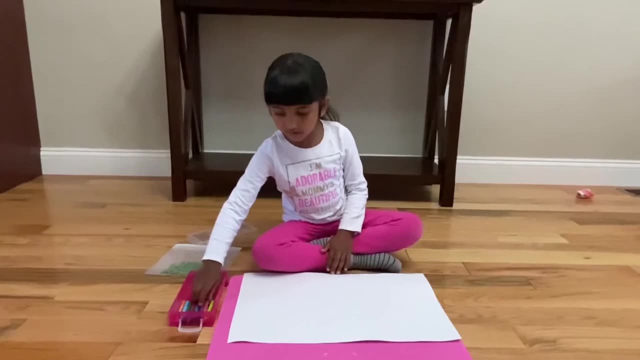 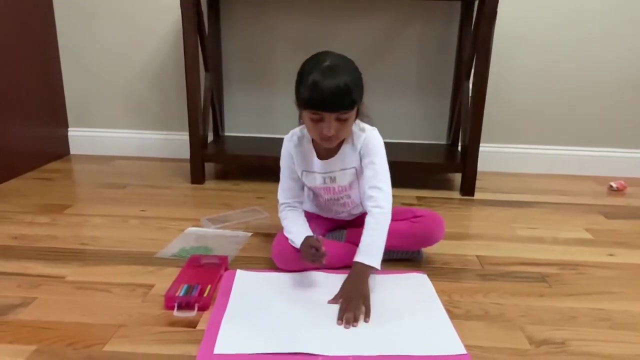 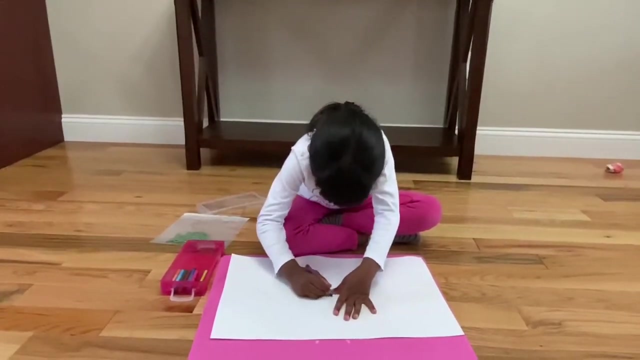 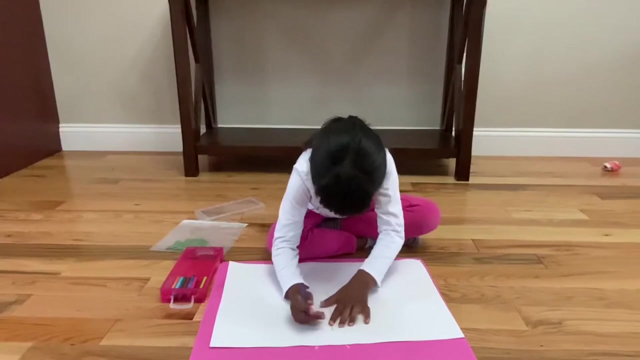 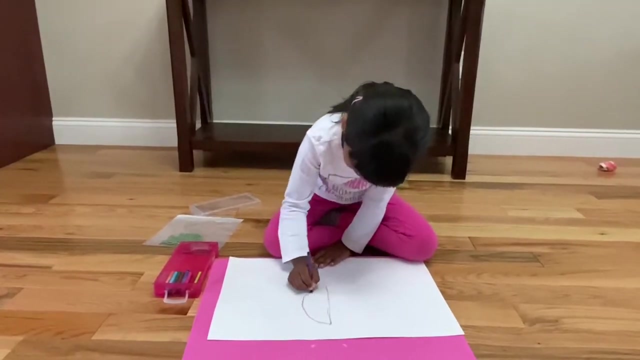 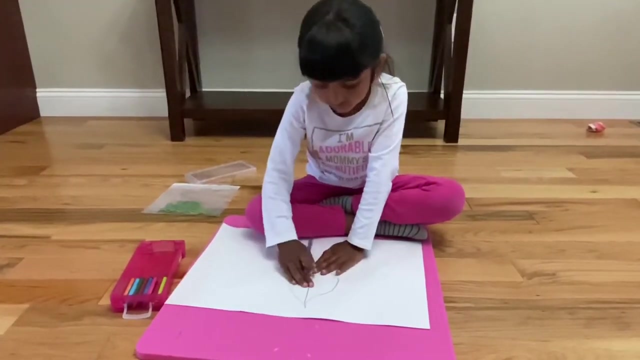 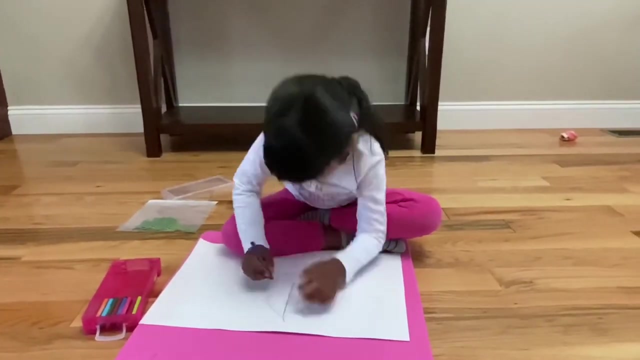 Opening the crayons. We're going to take purple. okay, Let's start. So I'm feeling the stem and tracing it, so it will be easy for me. Big leaf, I'm drawing the line Line up here, Okay, and I'm going to do the color so light. 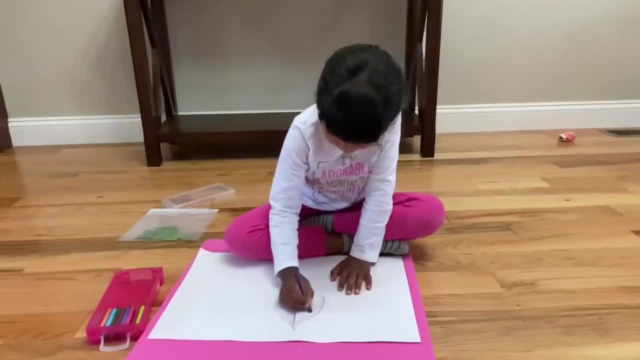 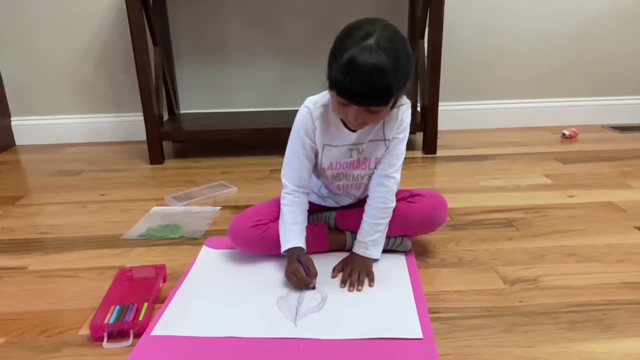 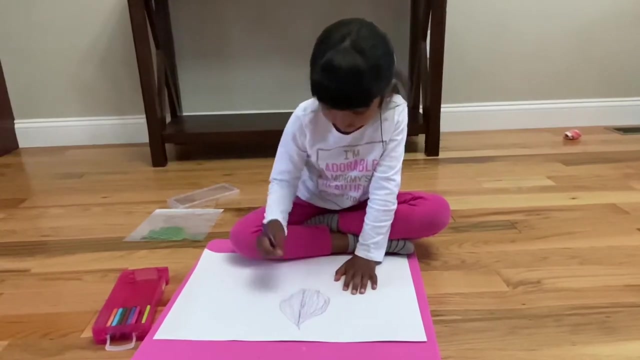 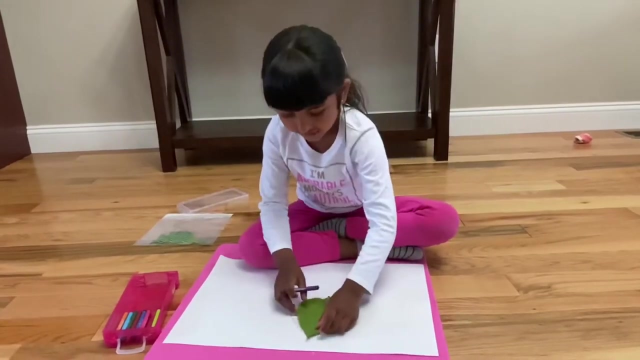 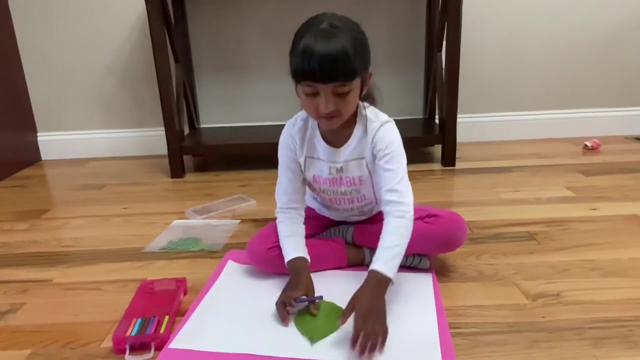 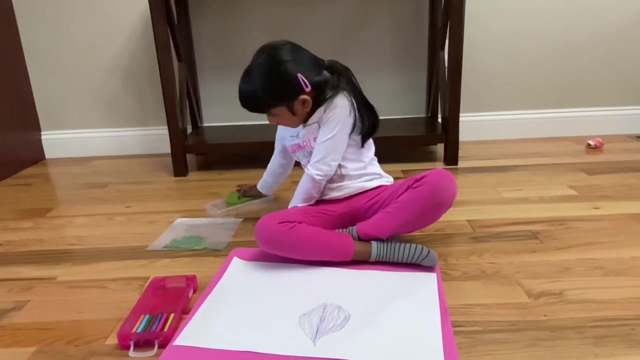 Like this, much Like this. okay, You don't want to be out the lines, right? So there you go. Your leaf is ready. The leaf that matches this: Ta-da Green. Next leaf, Next leaf. Let's put that on the paddle there. 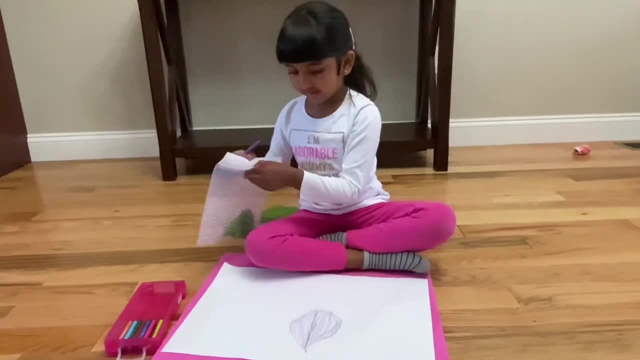 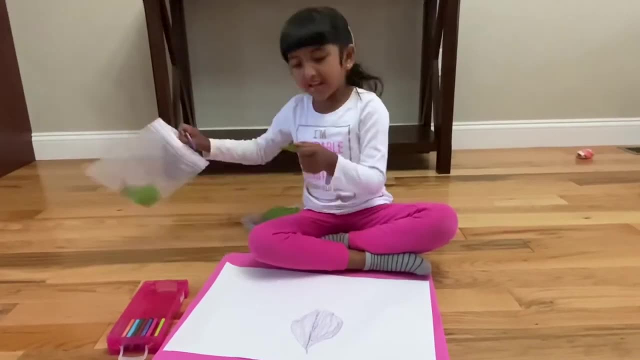 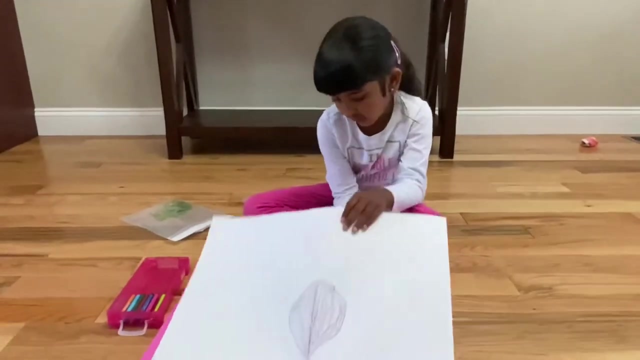 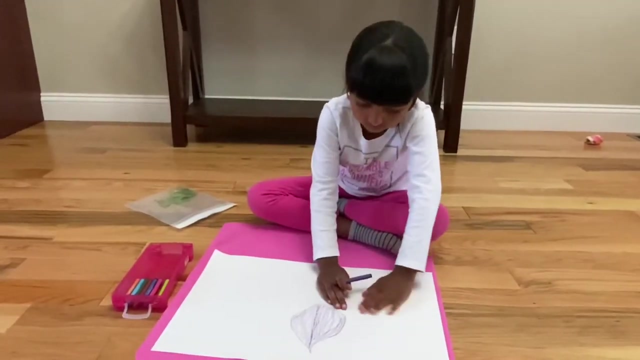 So next leaf we're going to write on the same paper. We're going to write the medium ones From here. I'll take it Okay, Ready, It's so cool. It's so cool, It's small. I got one different color that is smaller. 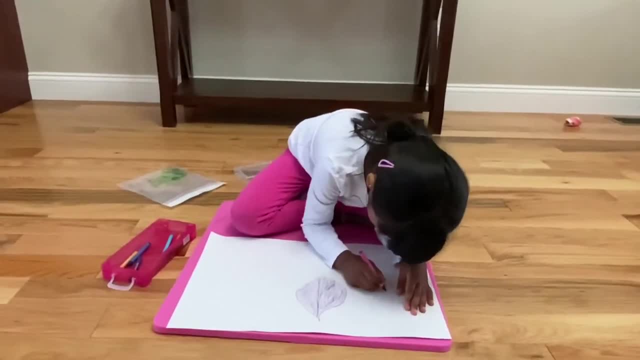 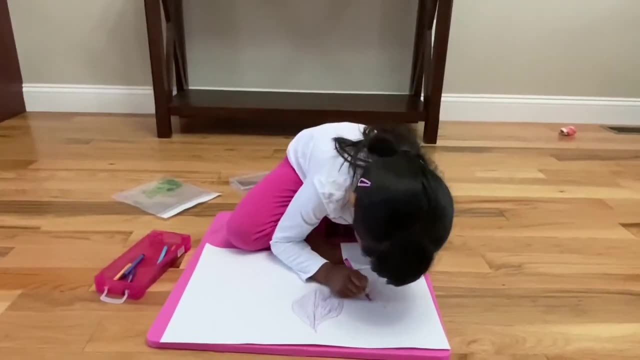 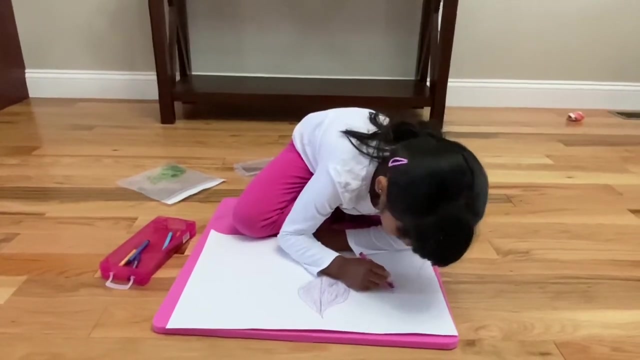 So let's trace it The top And colored it with the same color. Okay, So here's our leaf. Now let's take one more. I think I'll take this Boppy Bob, my eyes are closing. Let's put that over here. 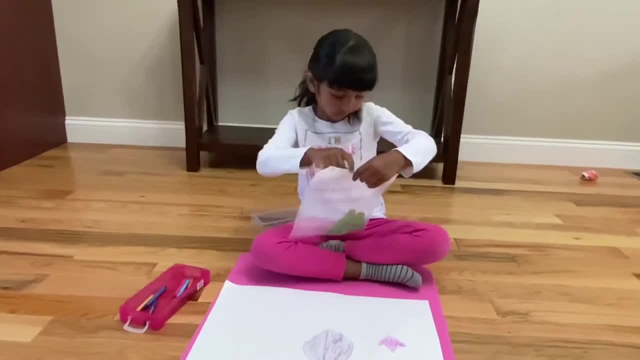 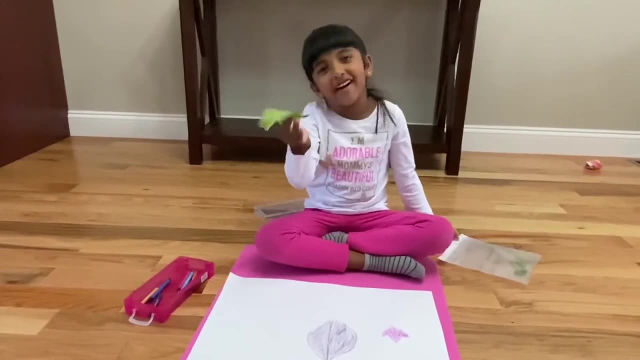 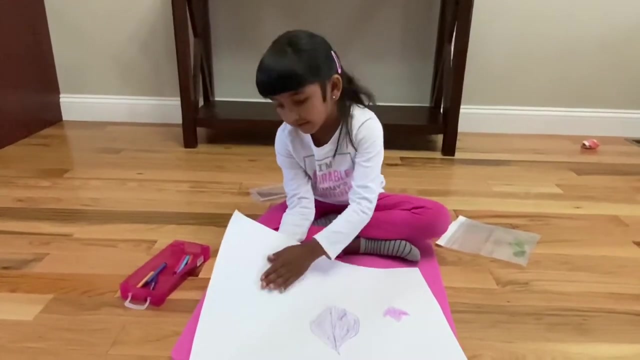 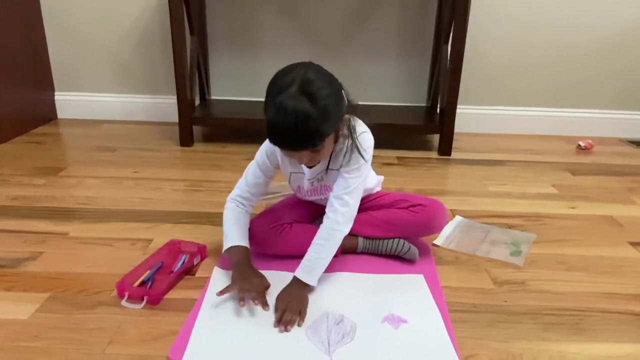 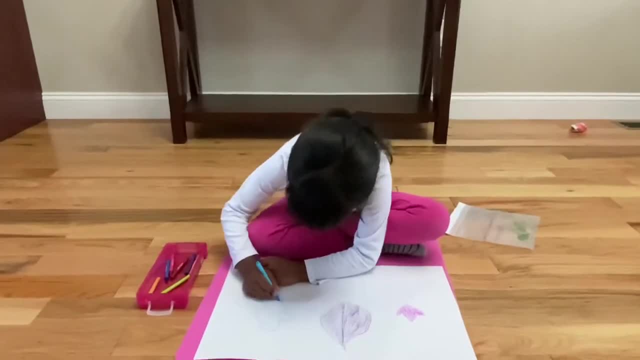 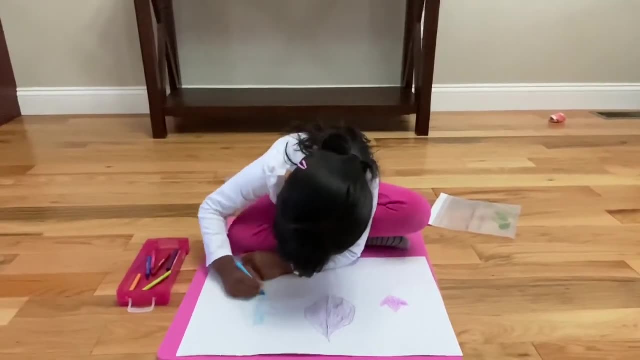 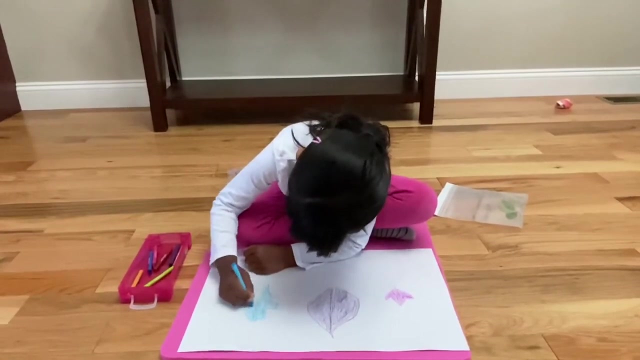 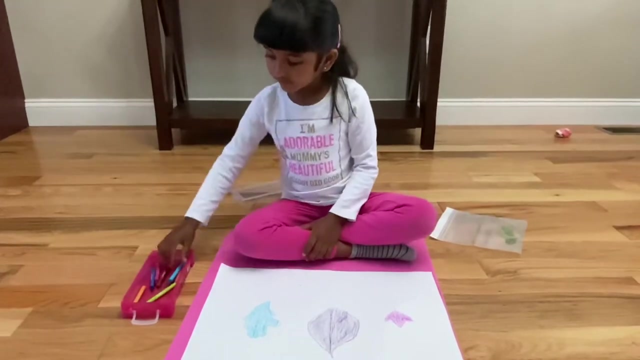 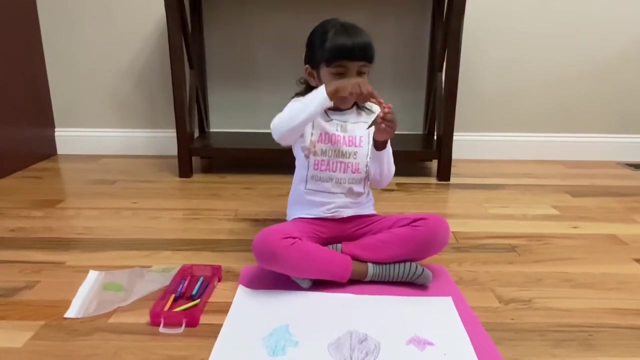 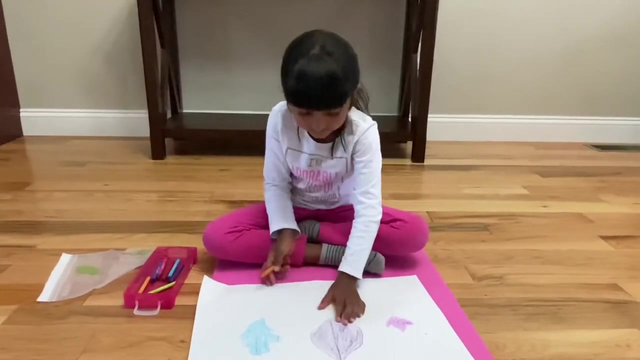 Okay, Okay, Okay, Okay, Okay, Okay, Okay, Oh, Okay, Hey, Alright, so the palette looks like this: Now let's do our summer flowers. Okay, Okay, Let's taste one more leaf: trace, trace, trace, trace-a-doh-ee. I'm gonna put that right there. 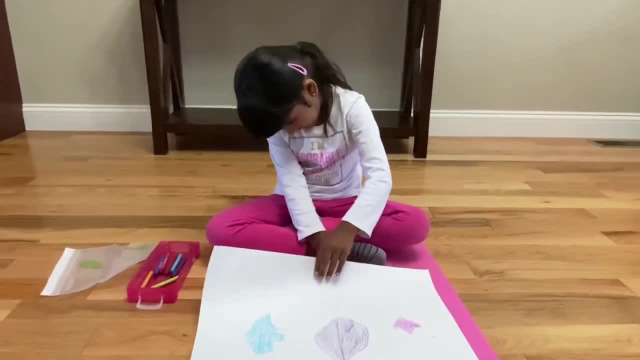 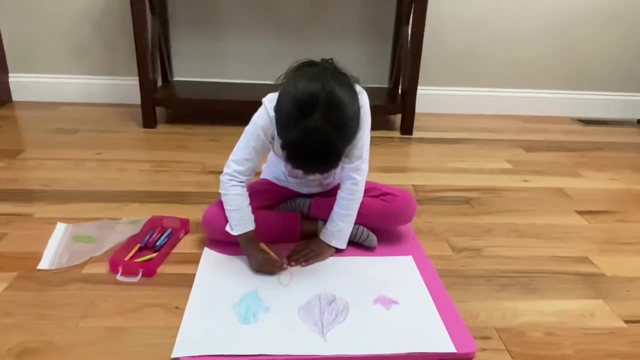 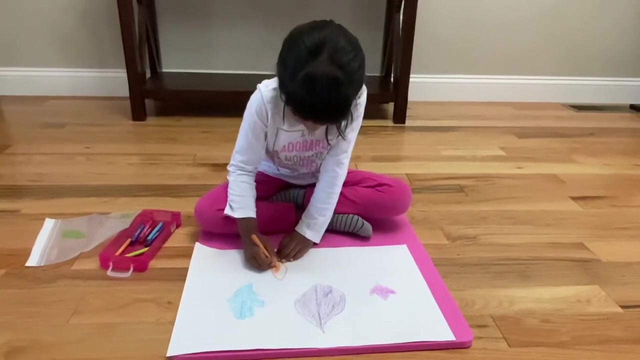 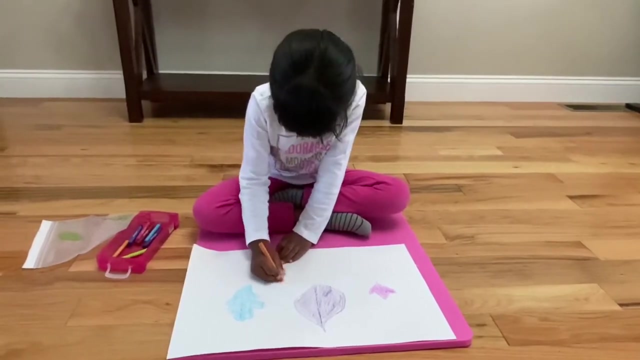 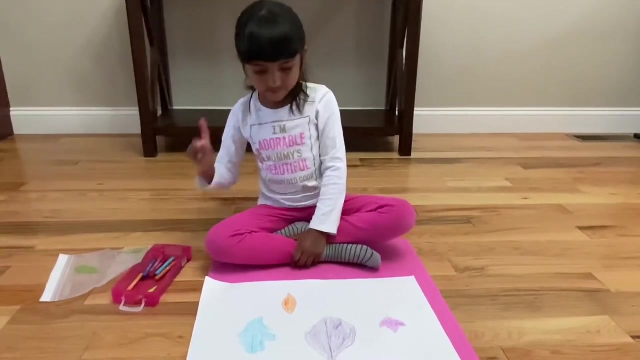 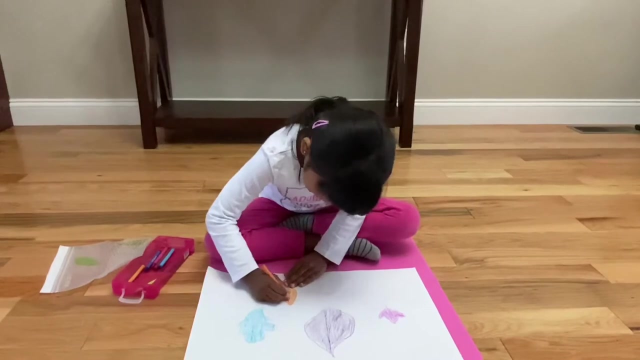 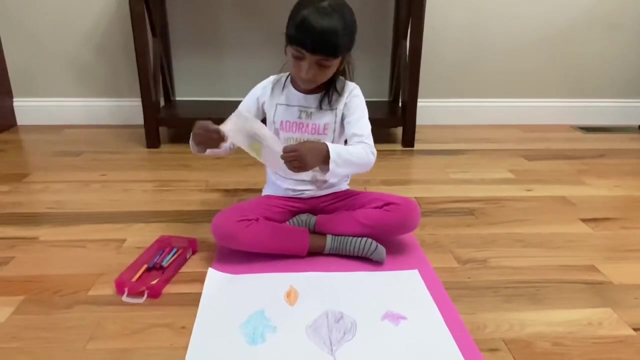 I'm going to color this orange. it's nice to color. do you like to color? Everyone likes to color. I like to color. One more leaf wet some top leafy green, leafy white. one more leaf I'm going to pick.